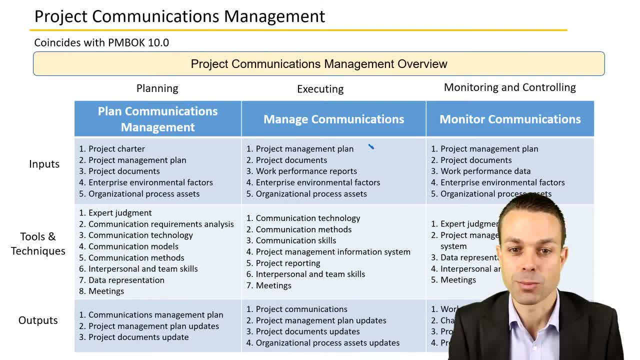 techniques and outputs that you'll see. We've got the project management plan, as always, and lots of project documents as well, And, of course, we've got work performance data and reports that are going to be an input so that we can see whether our communications are working as we want them to. 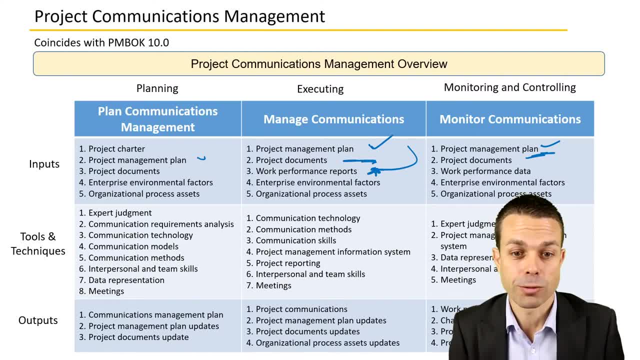 Now tools and techniques. you'll see a few new ones. So we've got communication technology skills and methods and, of course, different reports that we might see. We've got other interpersonal things like interpersonal and team skills, sometimes known as soft skills for your. 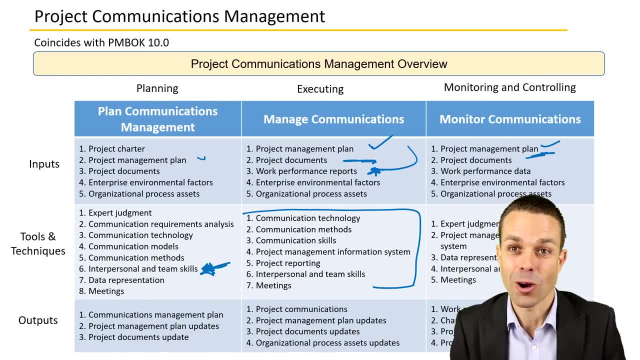 project, And these are really important things to hone over your project management career. And then meetings to tie everything together, which is a great and fast way to gather information from people or to disperse information across the project or your stakeholders in your project too. Now, of course, we've got things like project management plan. 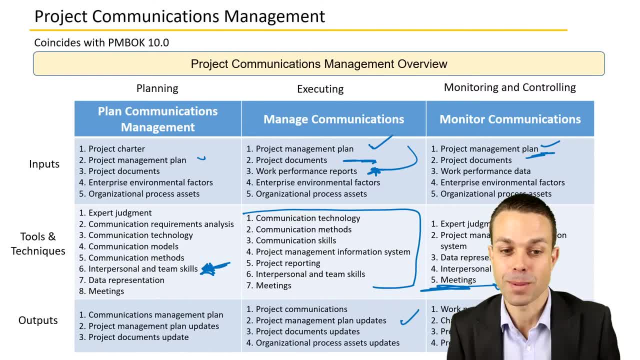 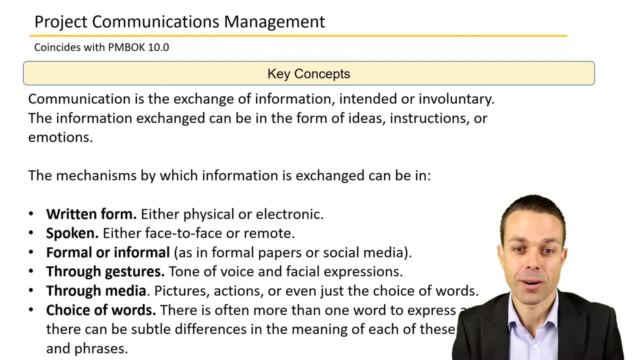 updates, maybe change requests that might come out of this if we need to make a change as usual and our communications management plan in how we're going to plan and proceed with all of the communications within our project. Key concepts for project communications management: There are a few. 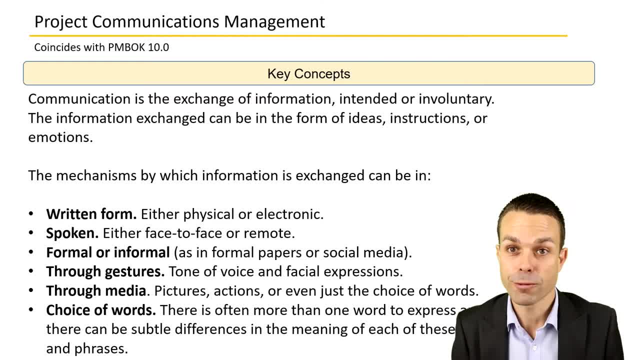 different ways that we can communicate. So it can be done in written form. so via email or letter or document or report, It can be spoken face to face or it can be over the phone. in this case too, Formal or informal could be an. 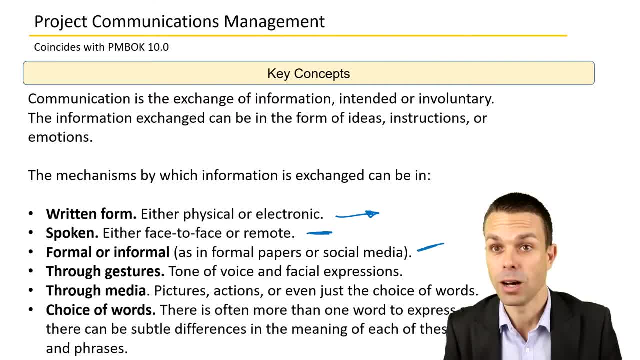 SMS, or it could be a formal document or a letter or a formal request. It could be through gestures now as well, so through tone of voice. If someone says yes, I'm going to get that for you right away. Or if someone says yes, I'm going to get that right, right away for you. 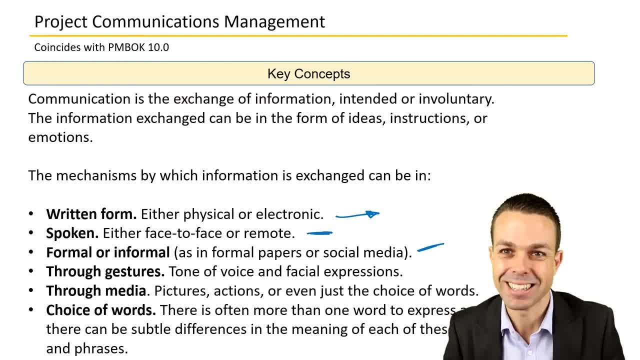 You know, there's a bit of a difference there and we pick up that change in the gestures or even facial expressions. So, through media, through pictures, actions of course, maybe memes or GIFs as well, So this is becoming more prominent. We might need to be communicating through those. 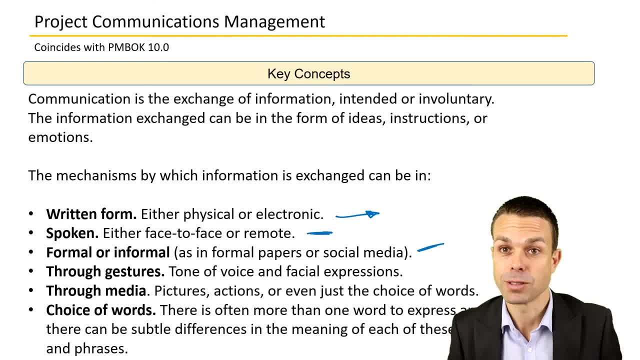 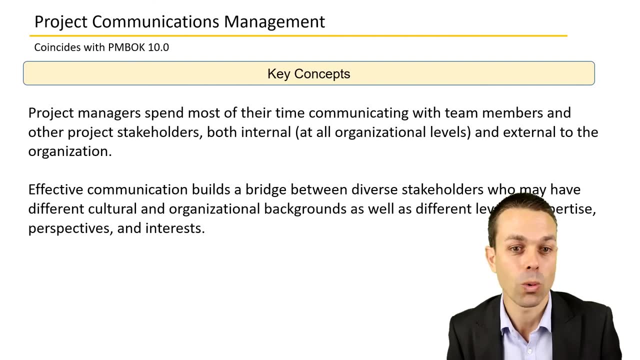 methods and choice of words, So sometimes the same word could express different ideas, and we just have to be aware of those subtle differences in the meaning of each of these words and phrases. Of course, project managers spend most of their time communicating in some way, shape or form. 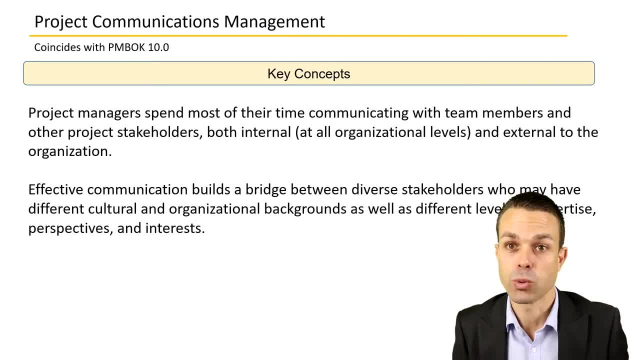 So effective communication builds that bridge between a diverse range of stakeholders. Maybe you've got many different areas in an organization needing to come together in order to create the deliverables for your project, And they don't usually work together, but it's your job as a 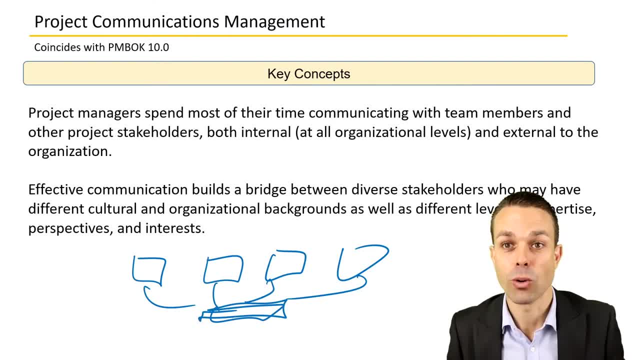 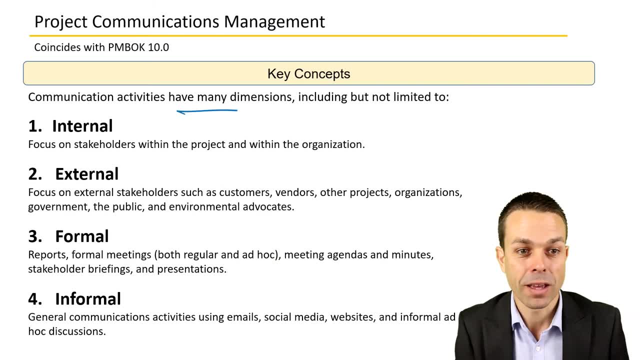 project manager to help facilitate and communicate between all of those parties in an effective way. Communication activities can have many different dimensions as well. We've got internal, where we're focusing on stakeholders within the project and within the organization. External might be external customers, vendors, other projects or organizations, maybe the government or public. 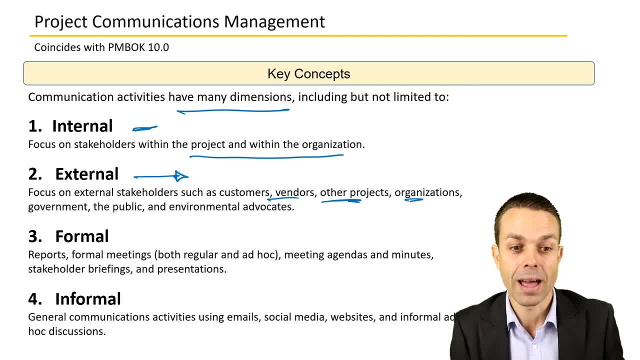 or environmental advocates. We might have formal and informal methods as well. So reports, formal meetings, meeting agendas and minutes might be formal or informal, might be just general communications, conversations by the water cooler, that sort of thing, or conversations amongst friends out of hours and that sort of thing. Other key concepts you'll see are hierarchical. 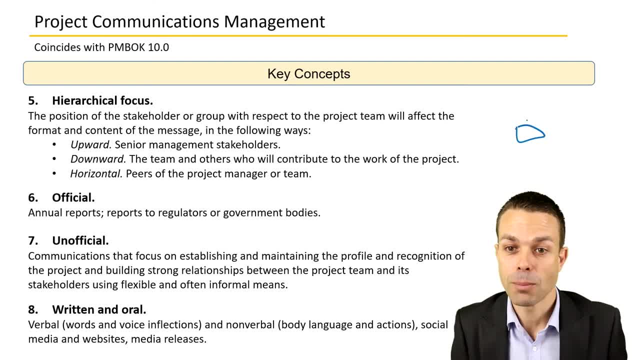 focuses. So, in other words, are you communicating up to senior executives, for example? Are you communicating across or horizontally to just your peers? So these are the people at the similar level to you within an organization- And are you communicating downward, as they say? 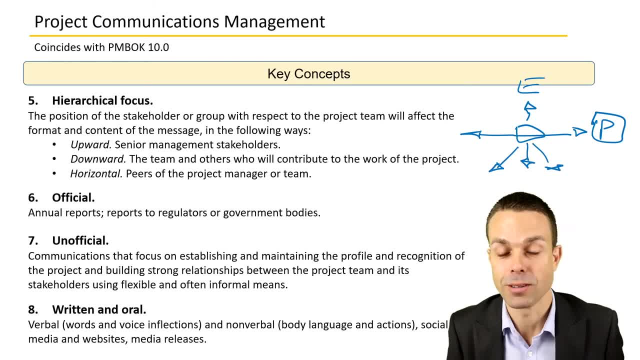 which is within the team that you're currently controlling, So the project team, And so this is all of the people who are contributing to the project work. So that's what we're looking at when we're saying communicating upwards, horizontally, or downwards, Official reports might. 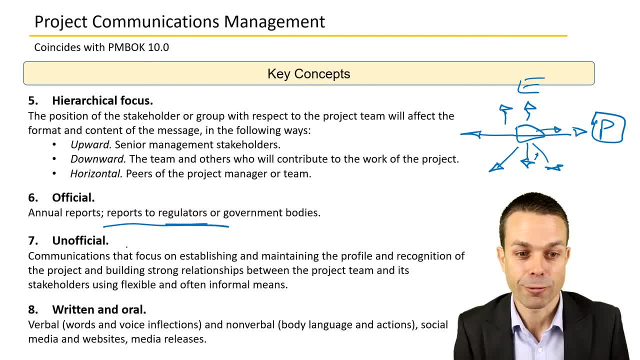 be seen: reports to regulators or government bodies, unofficial communications that focus on establishing and maintaining the profile or recognition of the project. So just building those unofficial conversations or communications- And there are written and oral, of course. So we might be saying something, there might be body language and or you might be writing something And as they, 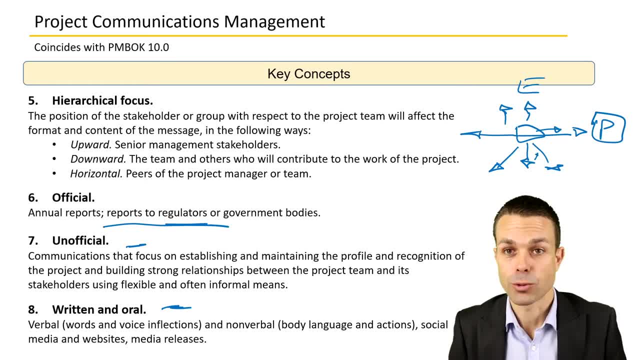 say. you know, the majority of what people pick up is through to voice tonation and also through expressions and body language. The actual words themselves often account for just a small percentage. I think around seven to 10% of the actual communication and getting 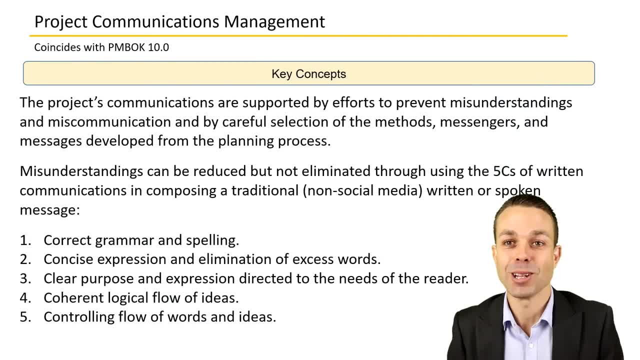 your point across. Misunderstandings can occur a lot when we're communicating as well, So it's something that we have to work on for ourselves and improve over time and also to be aware of. But reducing misunderstandings can be done through use of the five C's, So we've got correct grammar. 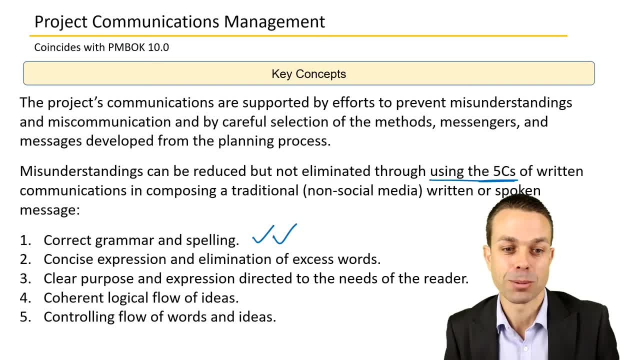 and spelling. Obviously that's going to help. It's going to reduce any miscommunication. Concise, so keeping it short and sweet where possible. Don't write a novel If you don't have to Clear purpose. So making sure you clearly have a purpose for what you're. 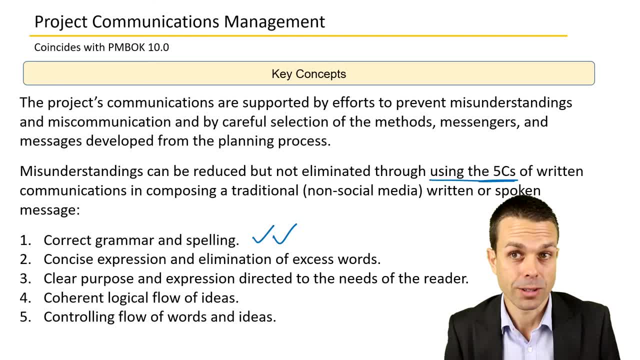 trying to express and an outcome. Not everyone does. And then you know those are the times when people tend to go off on tangents or waffle on Coherent and logical flow of ideas Based on. that again really helps with a clear purpose And controlling the flow of words and ideas. 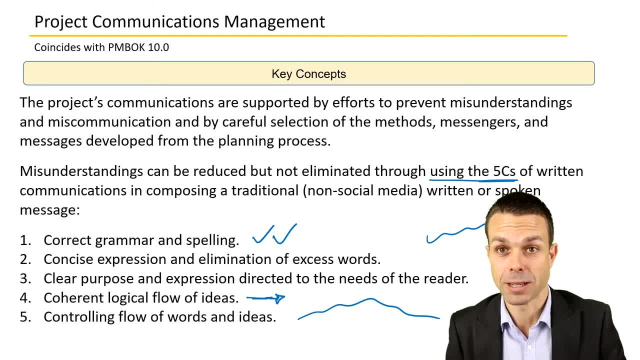 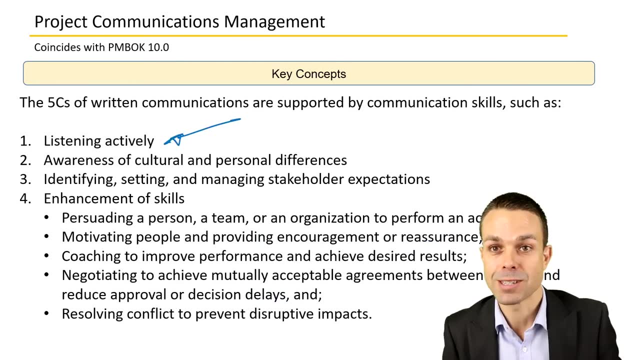 correctly. So again, not going off on a rambling tangent. if you can help it With a clear purpose and concise communication, those two things will help you a lot. The five C's are supported by things like listening actively, So sort of confirming with someone that you are understanding what they're. 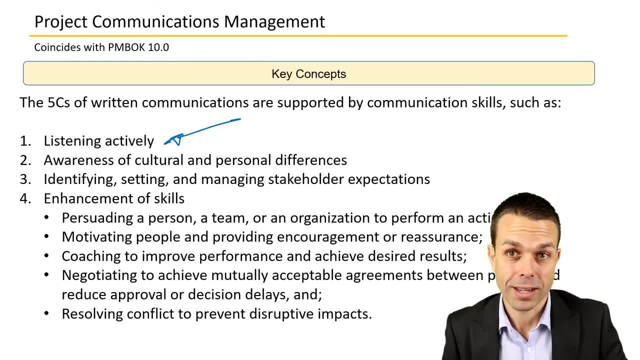 saying, reflecting it back to them, saying, OK, this is, this is what I hear you're saying. Is that correct? And then giving your point of view as well, Having awareness of cultural or personal differences, identifying, setting and managing stakeholder expectations upfront. So maybe not. 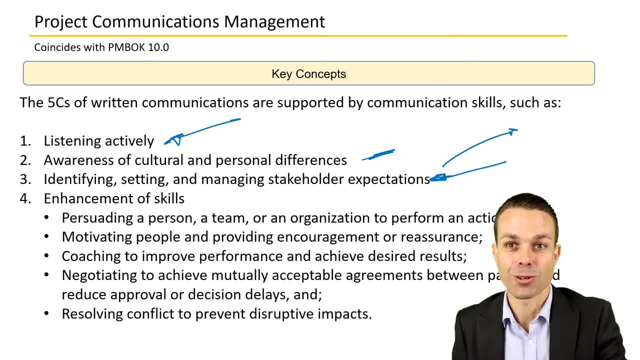 letting expectations get too wild so that you don't have to rein it back in later on. And, of course, enhancement of our own skills over time, Persuading people or teams or organisations to perform a certain way or an action. Motivating people to do the work, Coaching and improving. 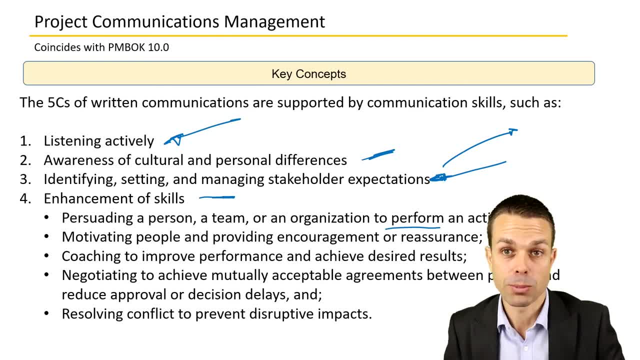 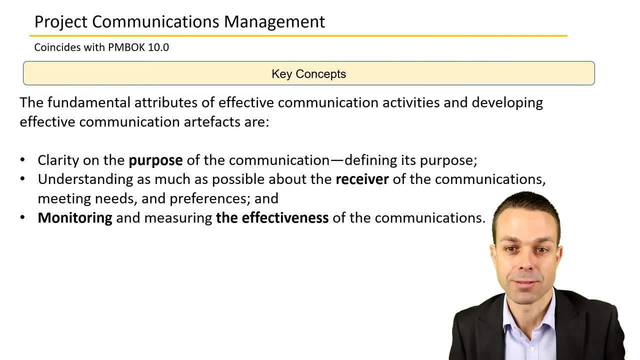 Negotiating between departments or projects or people to achieve mutually acceptable agreements between those parties And, of course, resolving conflict to prevent disruptive impacts to our project. So the fundamental attributes of effective communication activities and developing effective communication artefacts are: clarity of the purpose. 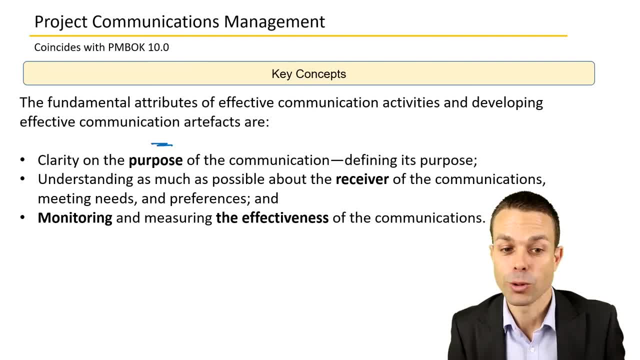 understanding as much about the receiver, so who you're communicating to, so understanding as much about them as possible, and then monitoring and measuring the effectiveness of those communications. Did you get your point across? If not, maybe we need to adjust our communication methods. 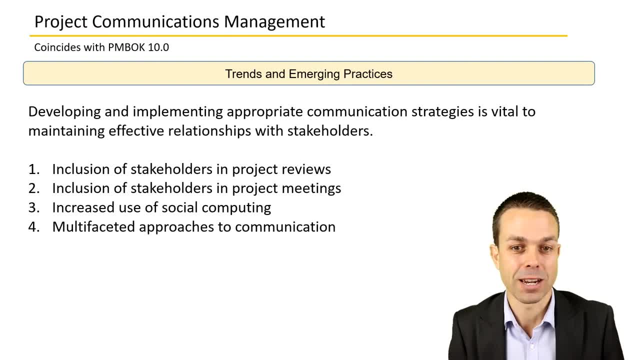 Trends and emerging practices we will see for project communications management. There will be a lot more including stakeholders in our project reviews to bring them on the journey. So we're much more into the whole team approach now, especially with the Agile approach. You'll see this a lot, But we want everyone to come along on the journey and including everyone. 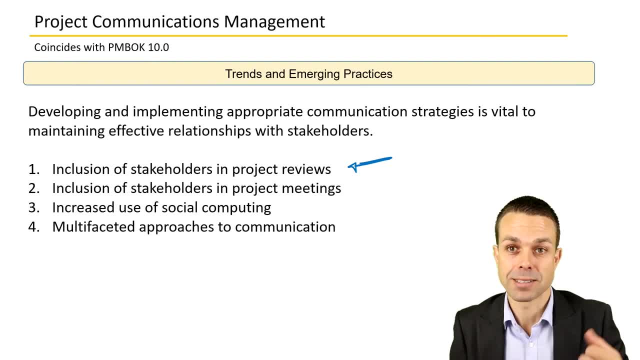 in those project reviews really can help with that. stakeholder engagement, Inclusion of stakeholders in project meetings for the same reasons. Increased use of social computing, so we might have Slack or Skype or even other social media channels that we can communicate through, And, of course, there are multifaceted approaches to communication because of that. 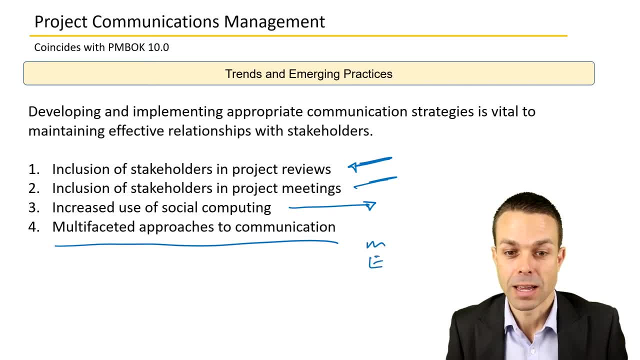 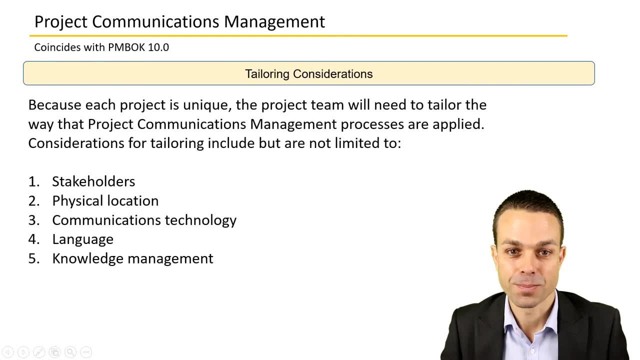 It might be messages, it might be emails, it might be on the phone, it might be face-to-face. So there are many, many, many different ways and we need to be aware of them all. Tailoring considerations for project management, for project communications management. 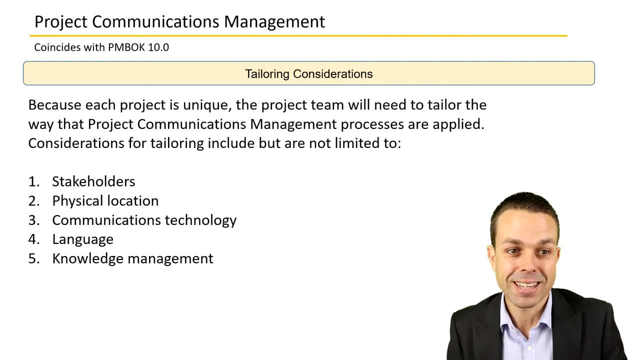 And because each project is unique, the project team will need to tailor the way the project communications management processes are applied. So considerations might include the stakeholders that we have involved. the physical location: Is everyone in the same place? Can we have daily stand-ups or do we need to have teleconferences, for example? 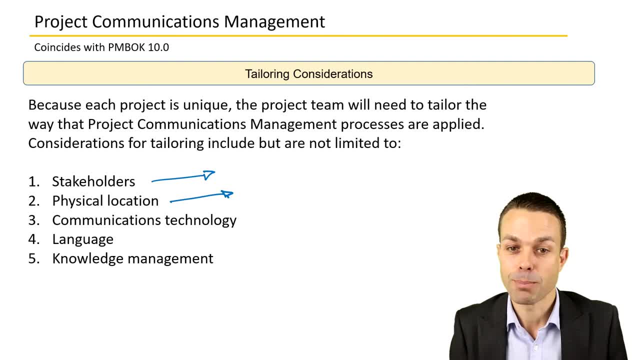 Are people in different time zones, And that impacts the communications technology that we're going to be using, the language that we're going to be using as well. And again, communication, It comes down to formal or informal language, as well as the cultural language that we're using. 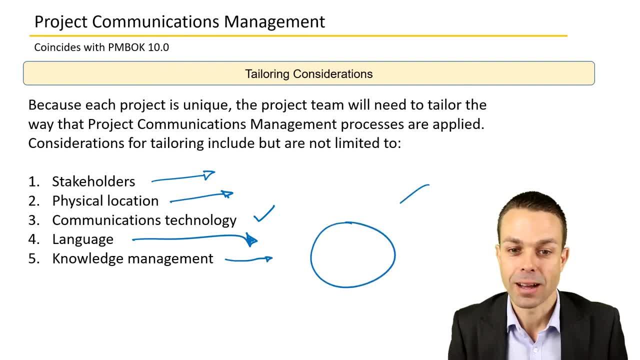 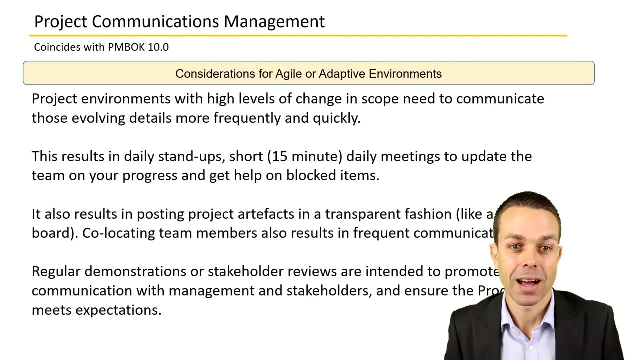 And, of course, knowledge management. How is everything gathered and placed into our project management knowledge information system? And then how is it dispersed and shown to everyone? as things change within our project Considerations for agile or adaptive environments, We might see. projects with high levels of change in scope might need to communicate those evolving details more frequently and quickly.